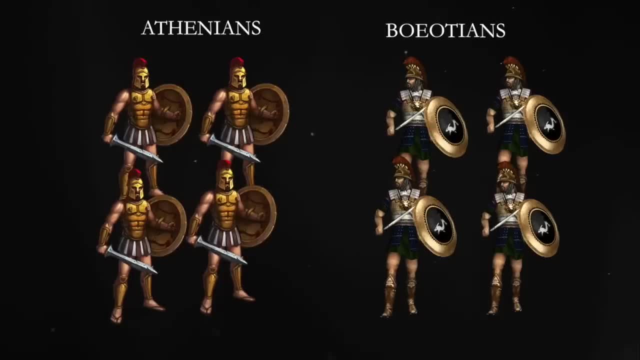 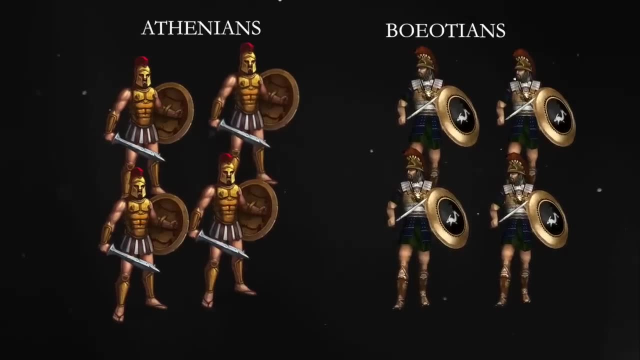 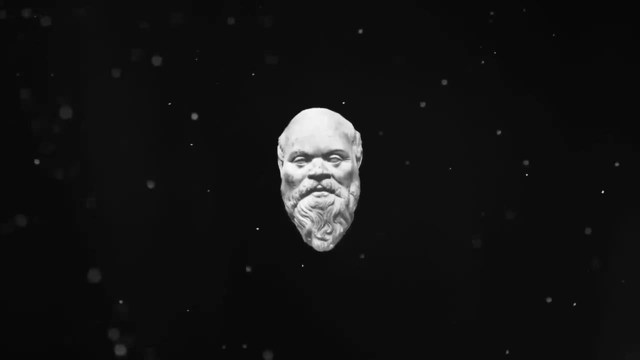 battle. Now imagine if all soldiers were to exhibit this very reasoning at the same time. If such an event would occur, they would all probably realize that they would be better off running away. This seemingly simple yet incredibly reasonable hypothesis is one of the first historical instances of game theory. Flash forward 2,368 years in 1944, Hungarian-American. 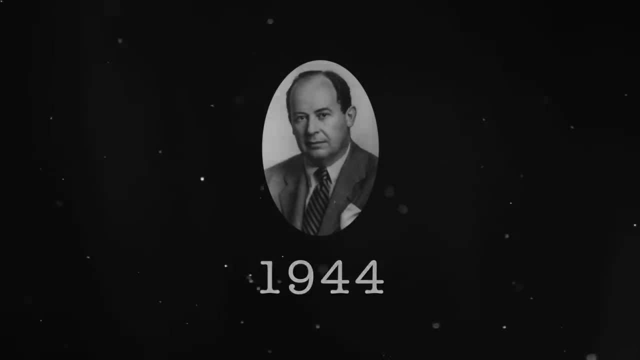 mathematician John von Neumann published a book titled Theory of Games and Economic Behavior. This foundational work contains the method for finding mutually consistent solutions for two problems. The first is the theory of games and economic behavior. The second is the theory of zero-sum games. This great book introduced game theory as a concept, thus extending its 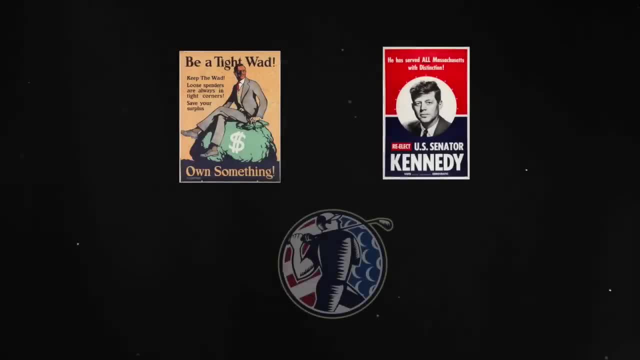 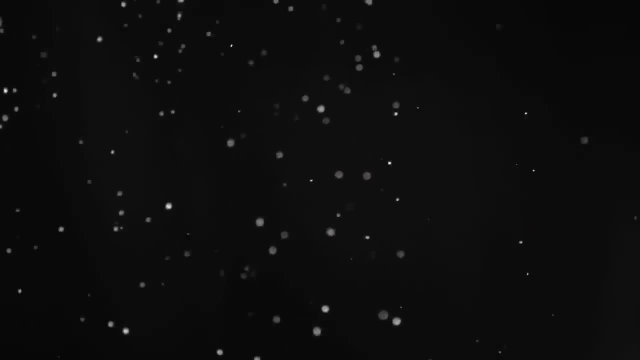 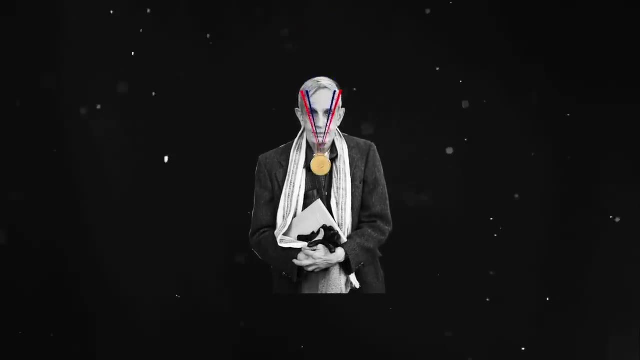 application to fields like economics, politics and sports, and leading to the expansion of the array of scientists that showed interest in it. One of those scientists was the legendary John Nash, who won the Nobel Memorial Prize in Economic Sciences in 1994 and popularized the idea of game. 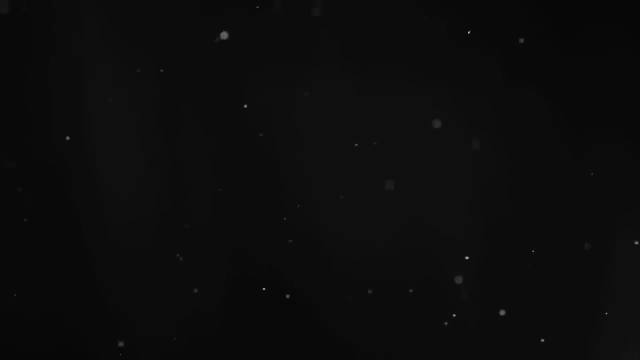 theory as we know it today. Something very fundamental about game theory is that it doesn't get its name from the preconceived notion of game. as we understand it, A game-in-game theory is an interaction between multiple people in which each player's payoff is affected by the decisions of others, Namely any single. 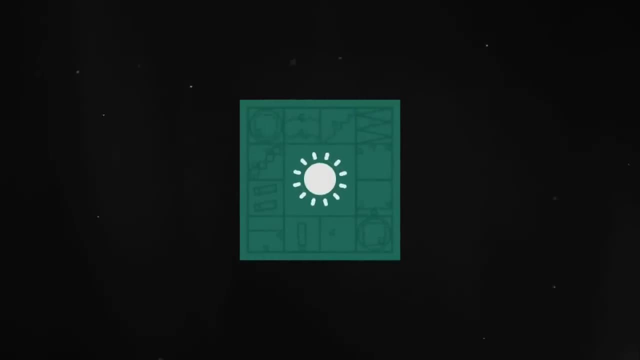 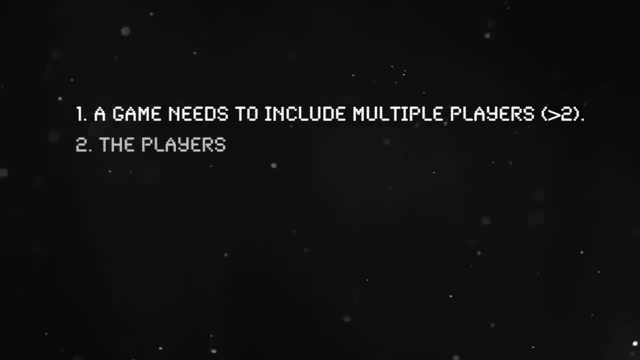 interaction you are part of can be analyzed with game theory in order to produce the most beneficial outcome. But before we get into the mechanics, let's lay out the main principles. Number one: a game needs to include multiple players. Number two: the players need to interact. 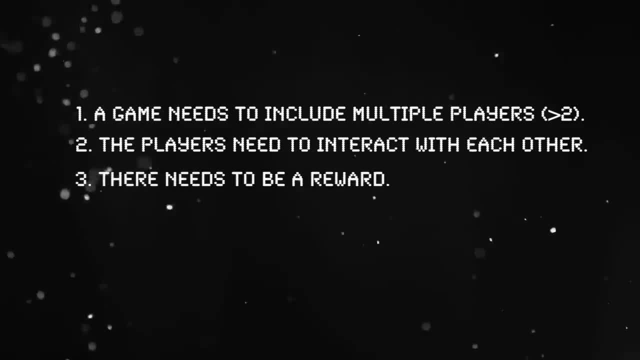 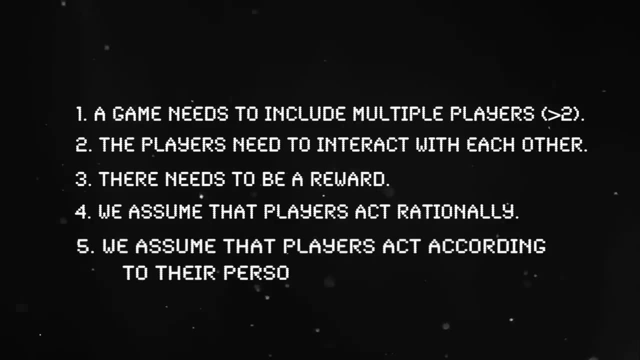 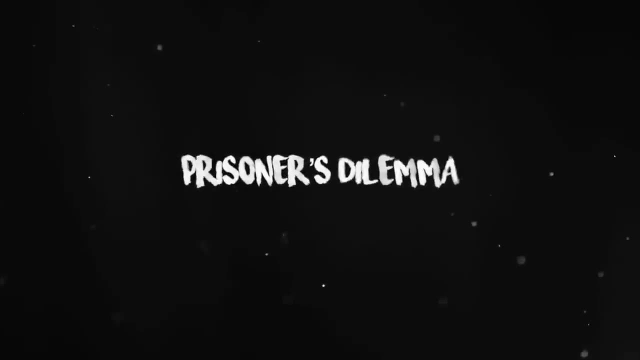 with each other. Number three: there needs to be a reward. Number four: we assume that players act rationally. Number five: we assume that players act according to their personal self-interest. Prisoner's Dilemma is the most widely mentioned game in game theory. The basic premise is how to 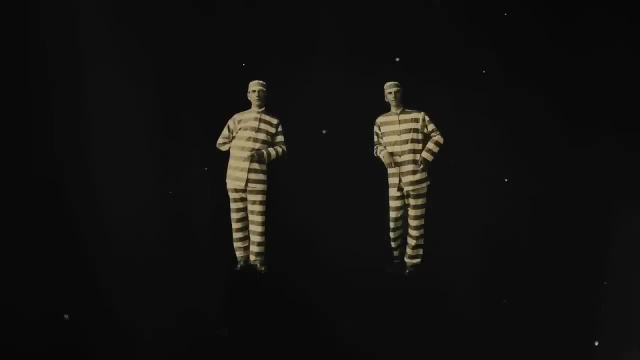 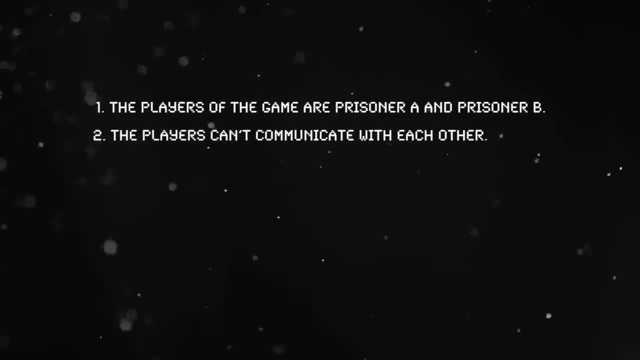 establish a mutually beneficial strategy between two members of a gang that got arrested and face potential imprisonment. The rules are as follows: Number one: the players of the game are prisoner A and prisoner B. Number two: the players can't communicate with each other. Number three: if A and B each betray each other. 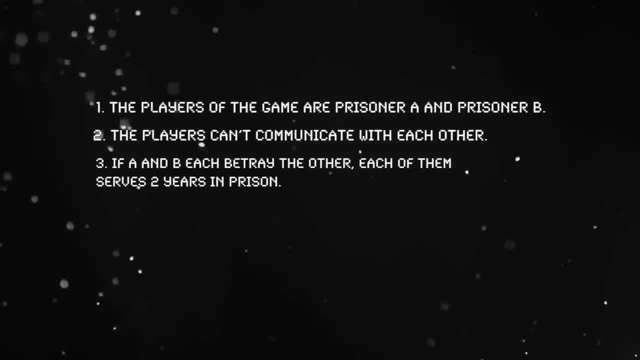 each of them serves two years in prison. Number four: if A betrays B but B remains silent, A will be set free and B will serve three years. And here is a quick list of the ways things expand Right now. here is how it works. Press because watch. it can't be handed. 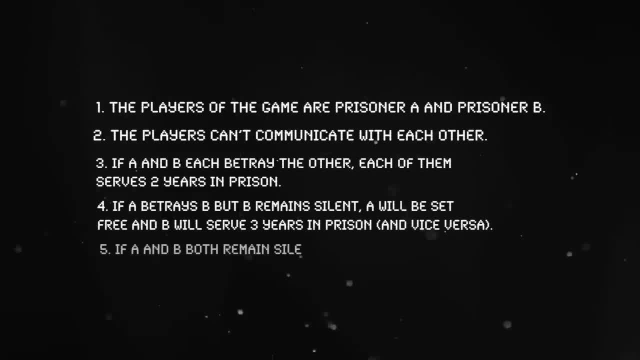 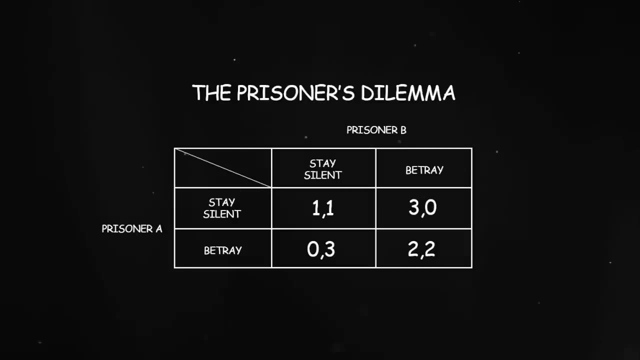 Roar years in prison and vice versa. And number five: if A and B both remain silent, both of them will only serve one year in prison. This matrix depicts the different choices of each member and signifies the number of years to serve according to each Prisoner's dilemma. exemplifies: 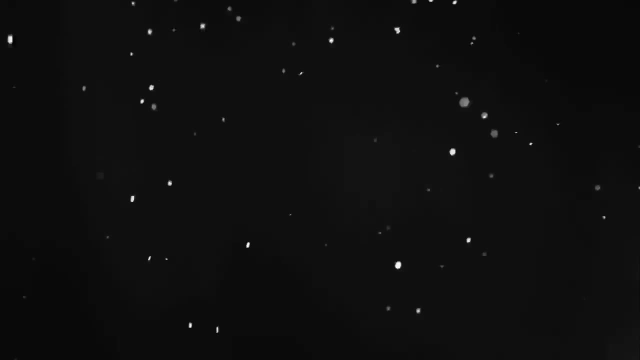 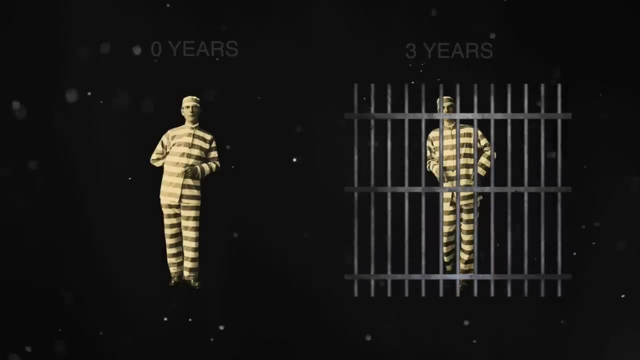 to a great degree, the substrate of human nature. The irrational, self-interest-driven gang member will most probably choose to betray his counterpart, thinking that he will get a better deal. This idiosyncratic choice will most certainly lead to a disaster for both parties. 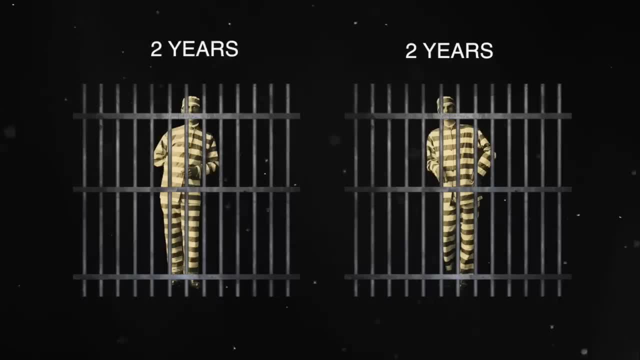 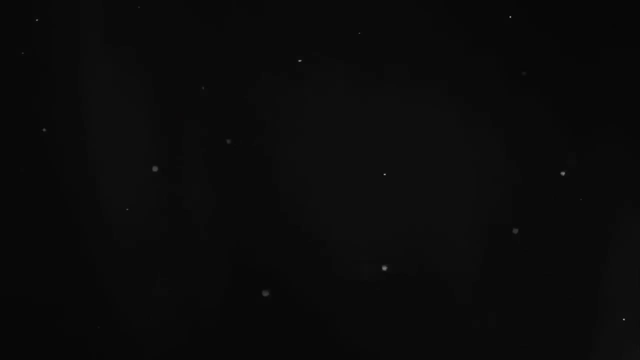 since they will get the worst deal possible. The obvious, mutually beneficial choice here is to keep silent. The main idea behind this game is to expose the inherent tendency of humans to display a lack of cooperation. in these and similar games, Game theorists usually coin the terms dominant strategy and Nash equilibrium to distinguish the kind of strategies followed. 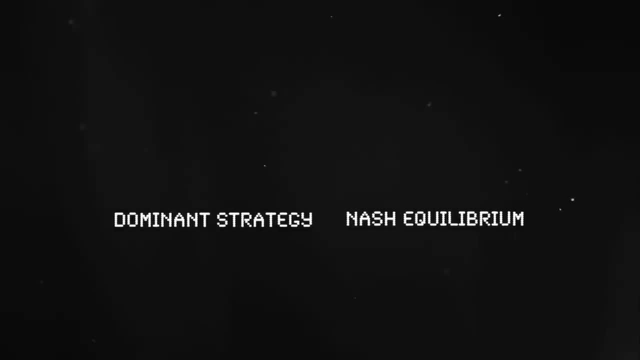 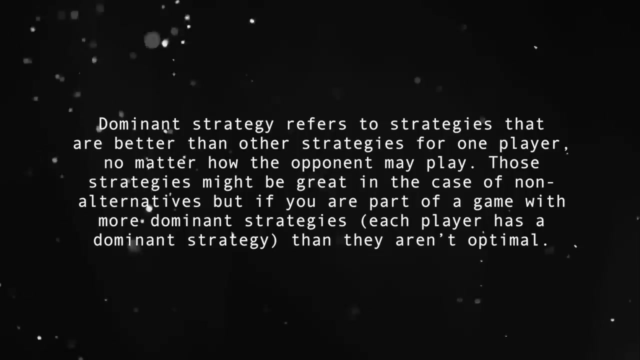 by the players. Those two terms are usually used together and form the basis upon which game theory is founded. Dominant strategy refers to strategies that are better than other strategies for one player, no matter how the opponent may play. Those strategies might be great in the case of non-alternatives, but if you're part of a game with more dominant, 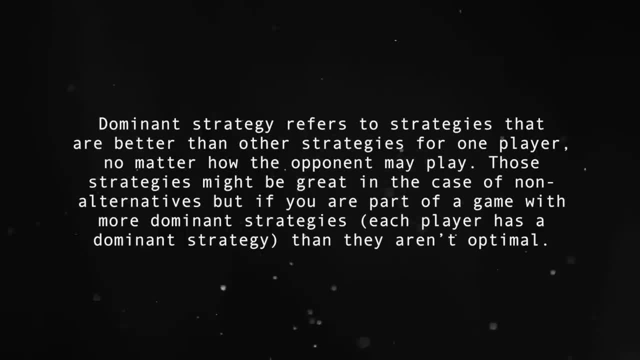 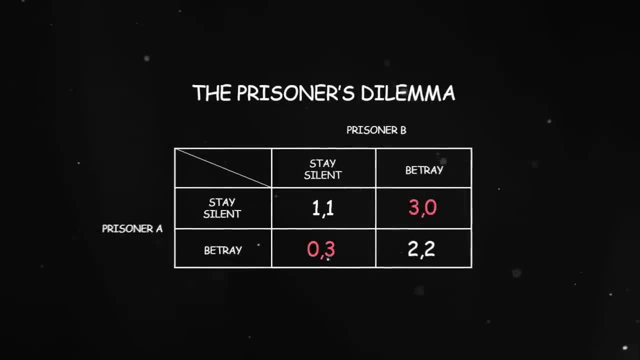 strategies, which means each player has his own dominant strategy- then they aren't optimal. In the Prisoner's Dilemma case, the dominant strategy for each player is to betray, And here is where the term Nash equilibrium comes into play. The term is used since John. 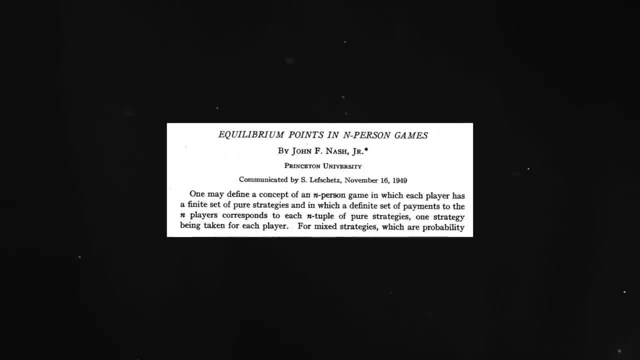 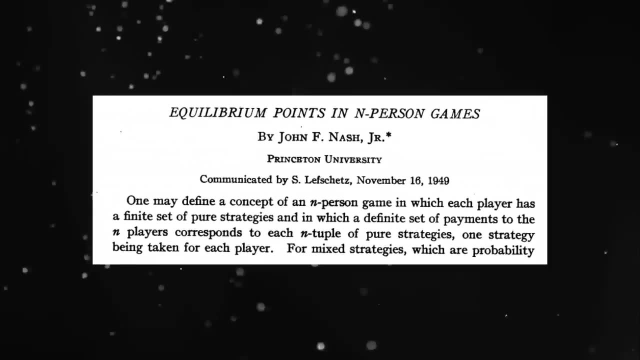 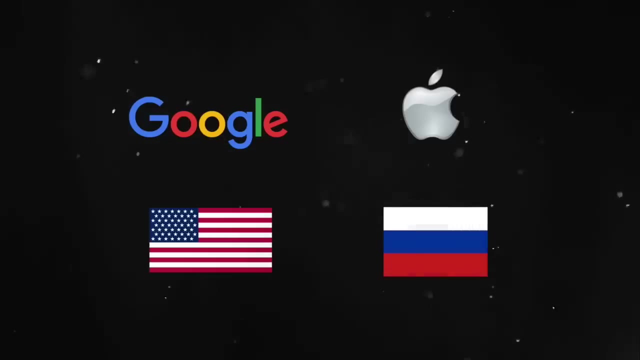 Nash explained the essentiality of equilibrium in his landmark work Equilibrium Points in End-Person Games. In essence, what he proposed is that even in high-level competitive games like Google versus Apple or USA versus Russia, there exists an equilibrium where no side 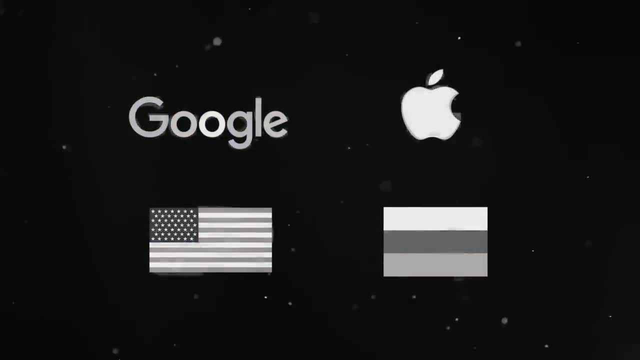 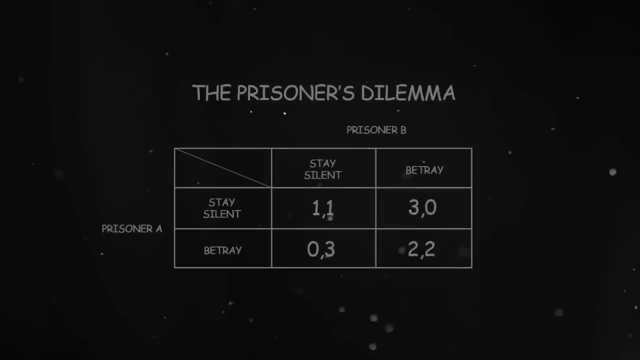 would benefit by changing its course. At this equilibrium, each side knows its adversary very well and sticks to its strategy. For instance, in the Prisoner's Dilemma, the Nash equilibrium is the upper-left square of the matrix, which means both prisoners. 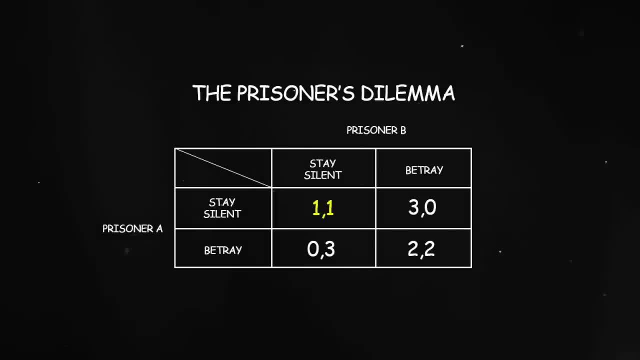 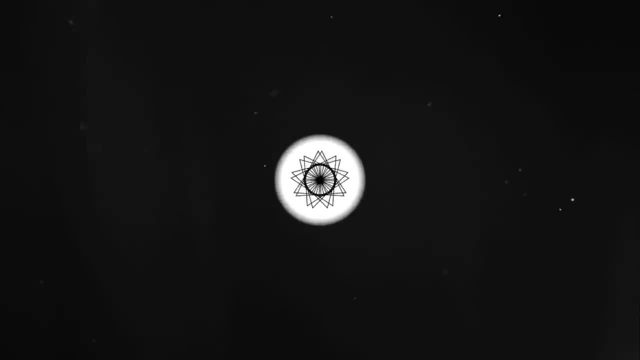 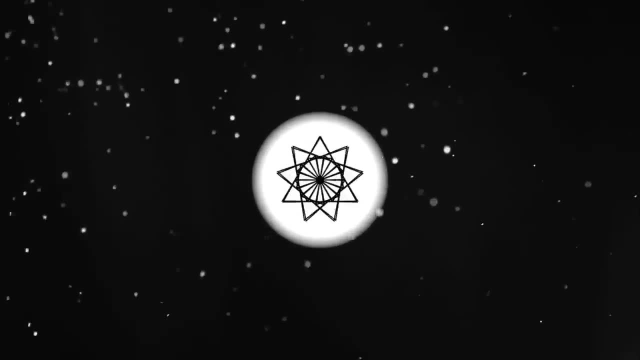 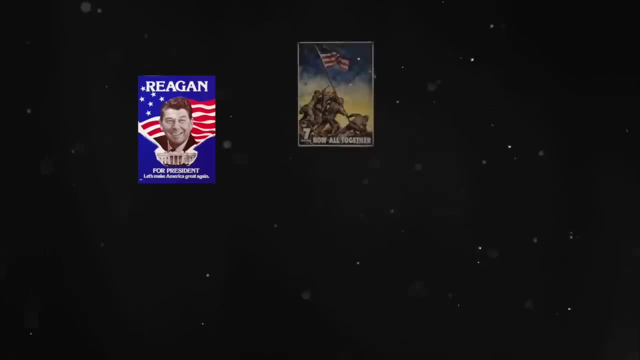 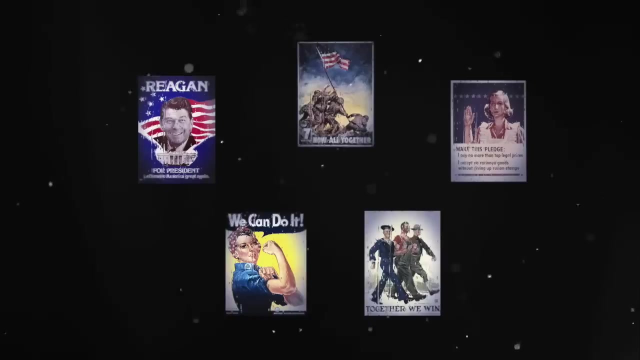 players will be better off trying to find it and form their strategy around it. This momentous revelation helped people in disciplines like politics, war, economics, business and social theory understand the world better and form better strategies. The inception of NASA Equilibrium was. 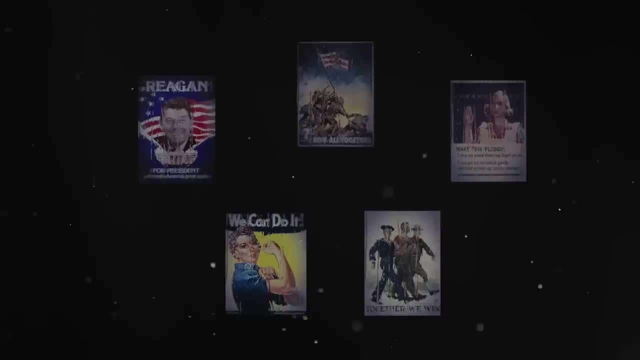 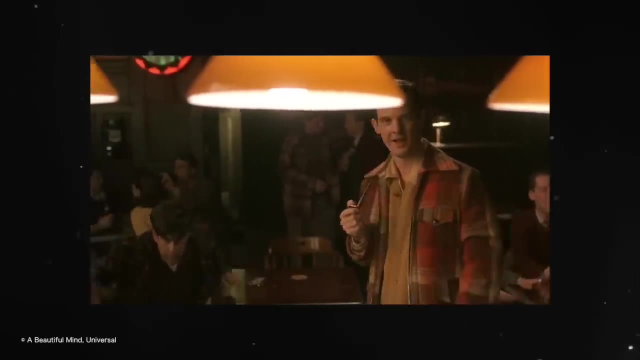 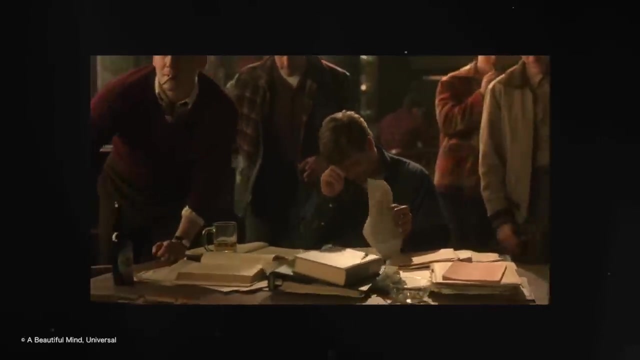 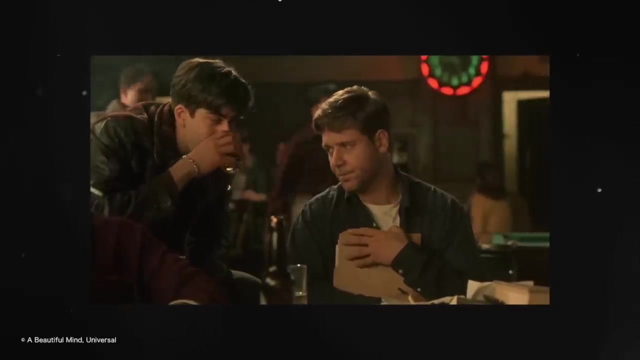 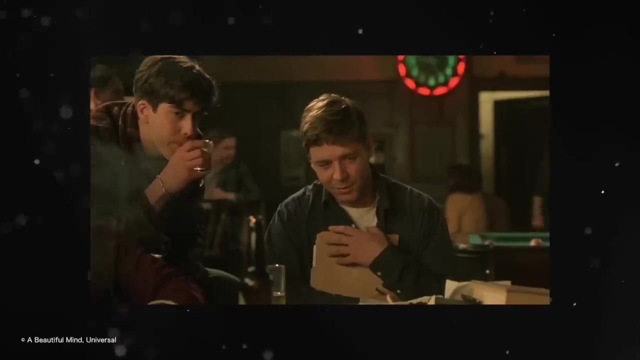 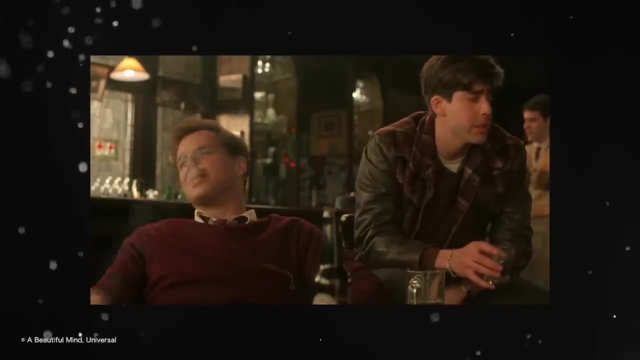 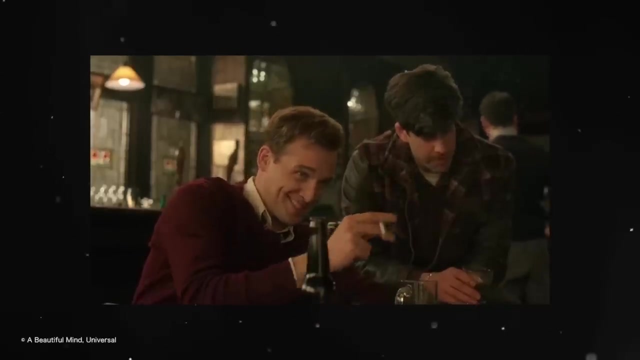 portrayed exceptionally in the wonderful movie A Beautiful Mind. Does anyone else feel she should be moving in slow motion? Will she want a large wedding? you think? Should we say swords, gentlemen, Pistols at dawn. Have you remembered nothing? Recall the lessons of Adam Smith, the father of modern economics. 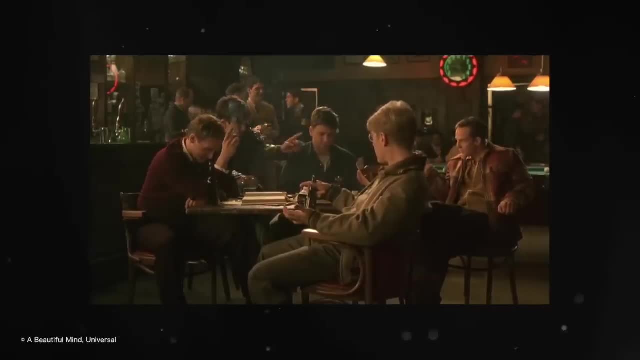 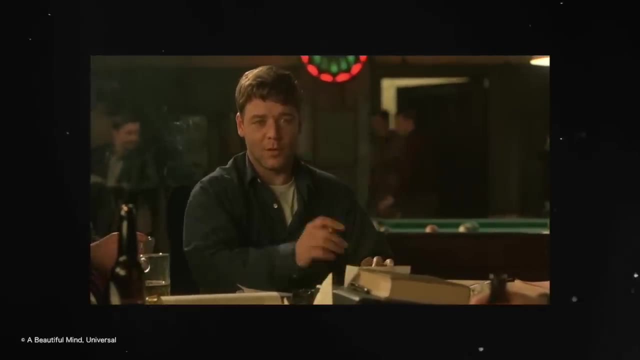 In competition. individual ambition serves the common good Exactly Every man for himself, gentlemen, And those who strike out are stuck with their friends. I'm not going to strike out. You can lead a blonde to water, but you can't make a drink. 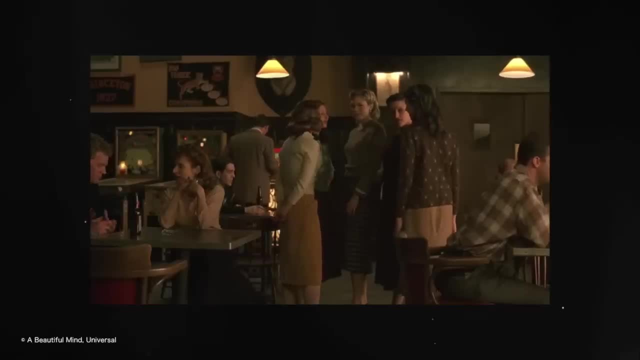 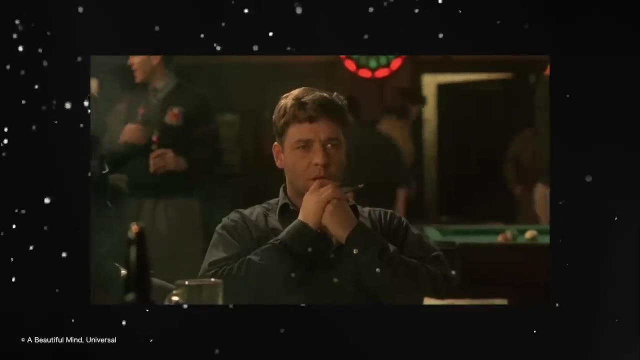 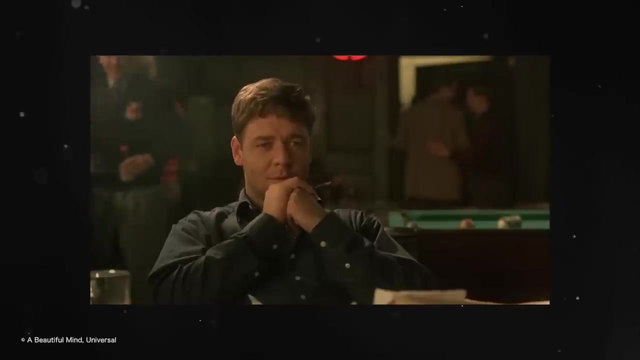 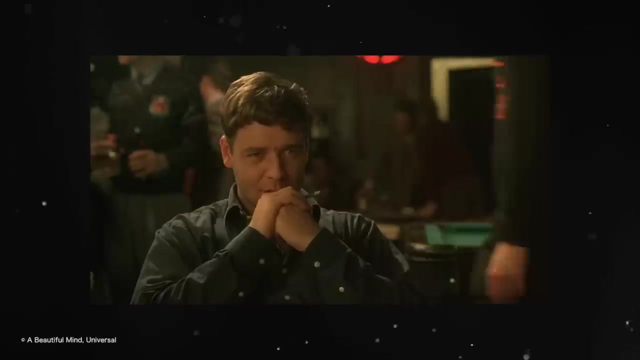 I have a plan. All right, nobody move. She's looking over here. She's looking at Nash, Oh God. All right, he may have the upper hand now, but wait until he opens his mouth. Adam Smith needs revision. What are you talking about? If we all go for the blonde? 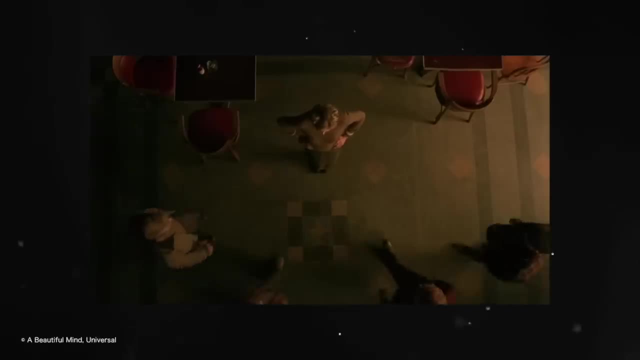 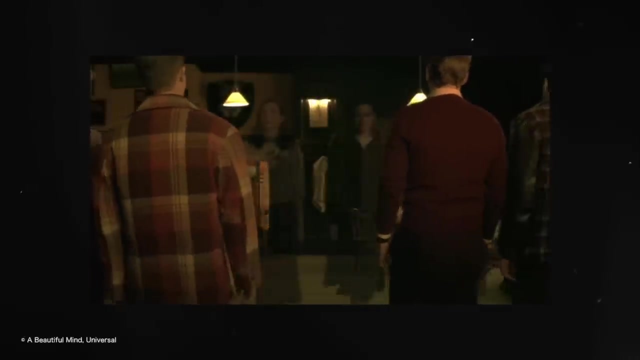 We block each other. Not a single one of us is going to get her. So then we go for her friends, But they will all give us the cold shoulder because nobody likes to be second choice. But what if no one goes for the blonde? 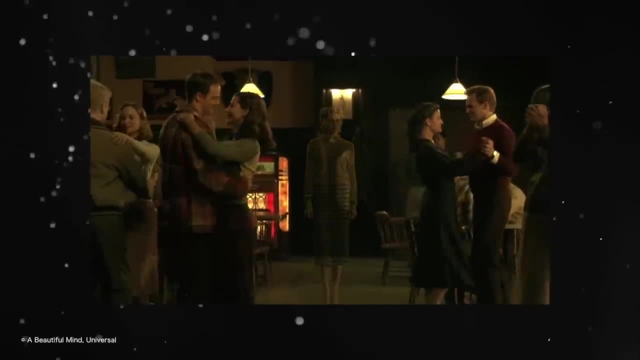 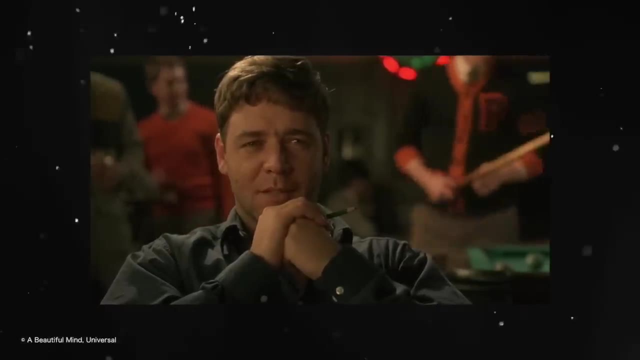 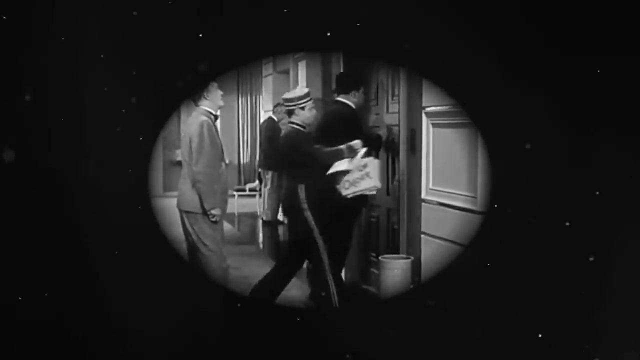 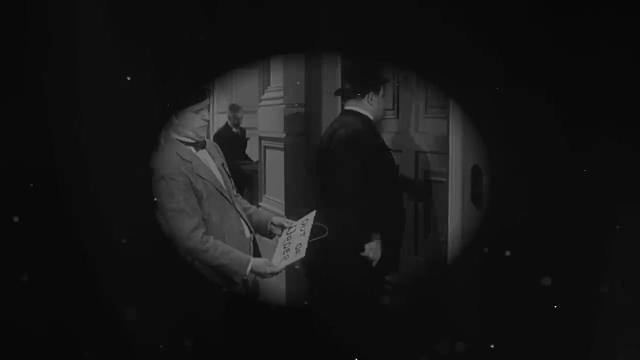 We don't get in each other's way and we don't insult the other girls. That's the only way we win. That's the only way we all get laid. Even if people or companies rationally follow their own self-interest, the best outcome is hard to reach when they can't or don't cooperate. 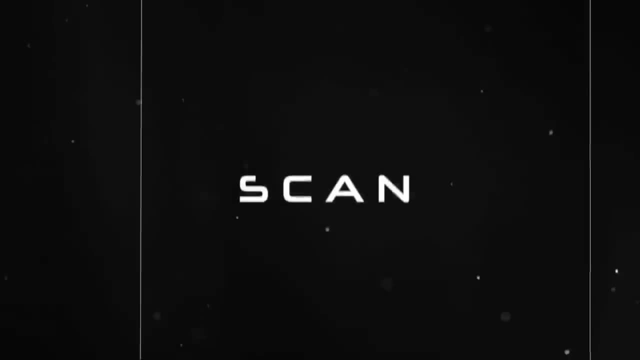 Therefore, the best strategy is to continually scan the market for potential alliances. People who can forge strong alliances will eventually become part of oligopolies and thus dominate their market. The rest will consequently be ostracized. That's what I love about game theory: It approaches the game of life from its most. 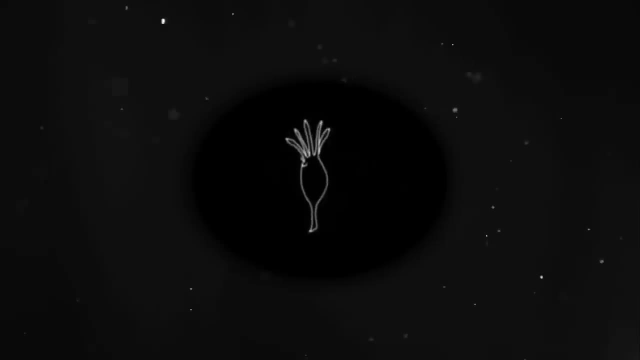 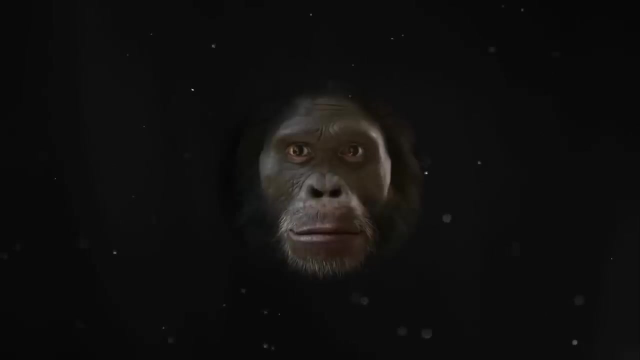 axiomatic principle, That of evolution. Evolution equals adaptation, and therefore life is an omnipresent game of adaptation. Humans thrive in cooperation because it is the main strategy that helped us survive and thrive after years of adversity and strife. It is an omnipresent game, but its main strategy is to fight the battle. 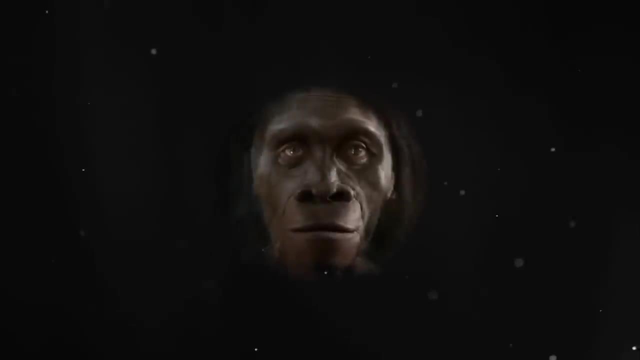 to fight the battleитуcom, to fight the battleuzucom, to fight the battleuzucom, to fight the battleuzucom. struggle to compete against different forces of nature. The sad thing is that, after establishing our sovereignty, we overpowered other species and, in most occasions, nature itself. but 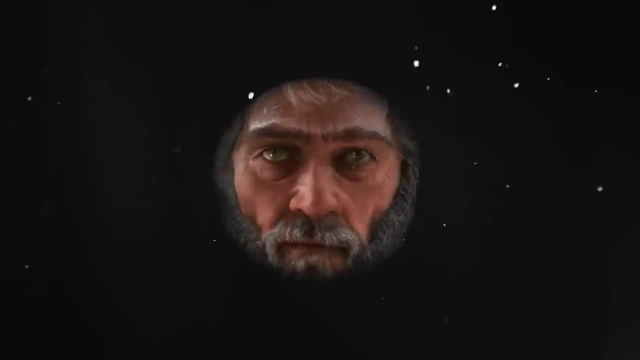 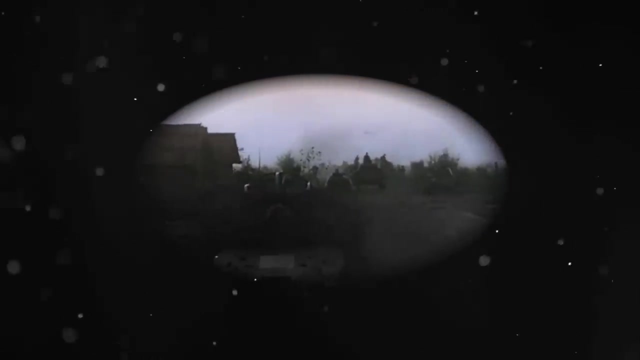 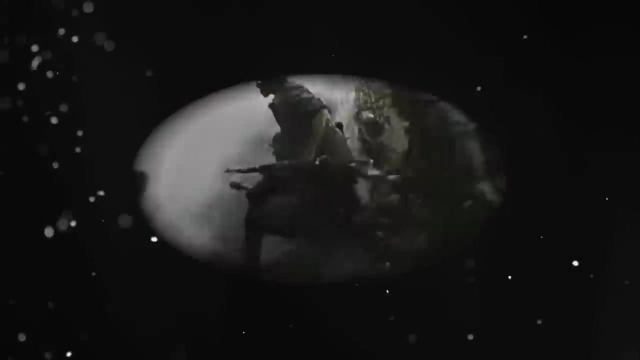 eventually, we turned ourselves against each other. There are a variety of factors that affect the descent to the point we have reached, but a game theory mindset can work to our advantage. I always believed that chains and equilibrium start at the micro level, And that is something we fail to grasp because 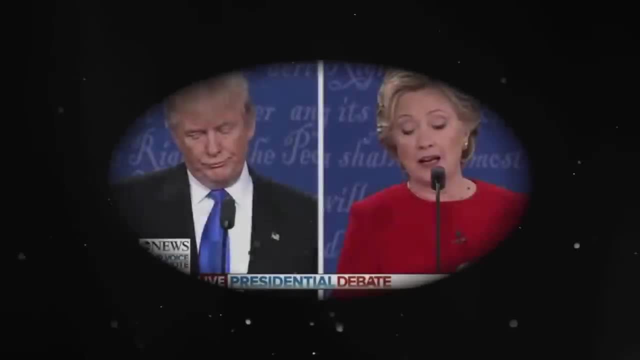 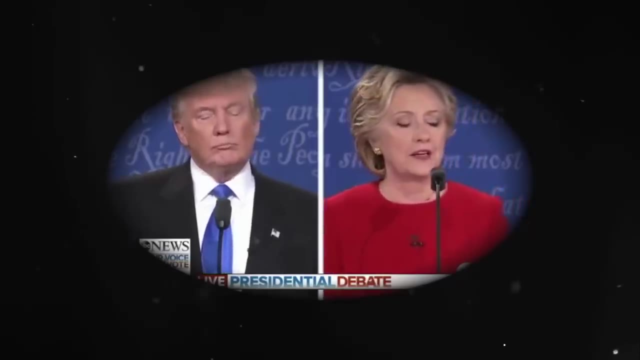 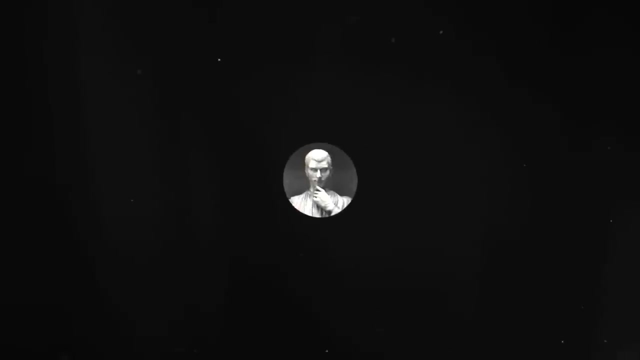 we are usually consumed by events. at the macro, It is interesting to be in the know and discuss and argue about politics and national strategies, but at the end of the day, the trigger is pulled by the respective strategists. What each of us could do instead is to use game. 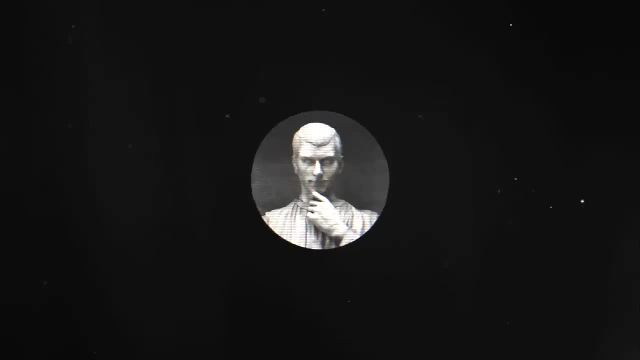 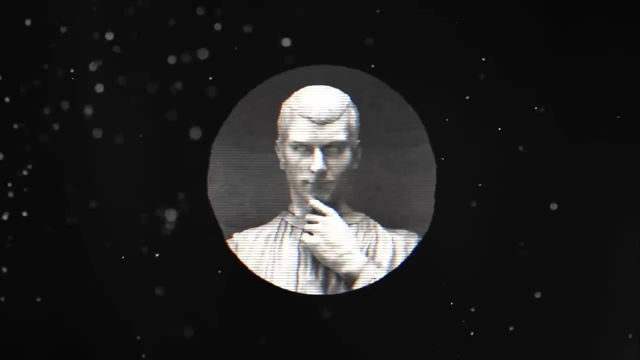 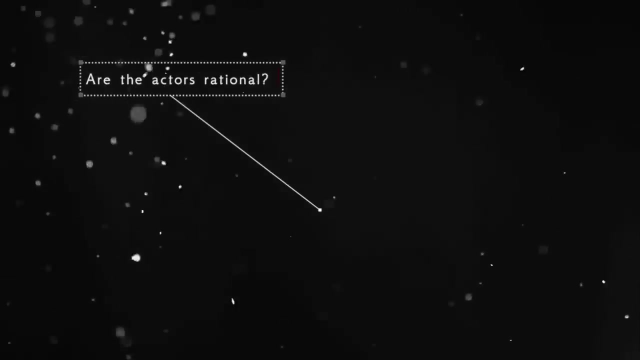 theory in our most challenging decisions and our closest relationships. So let's start. Regardless of what decision you have made and how this will impact your future, think like a game theorist. Ponder questions like: are the actors in the situation rational?